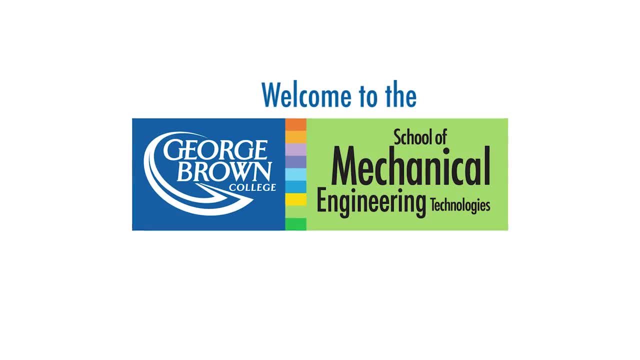 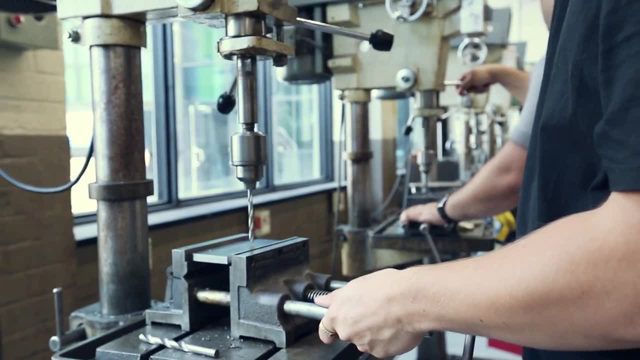 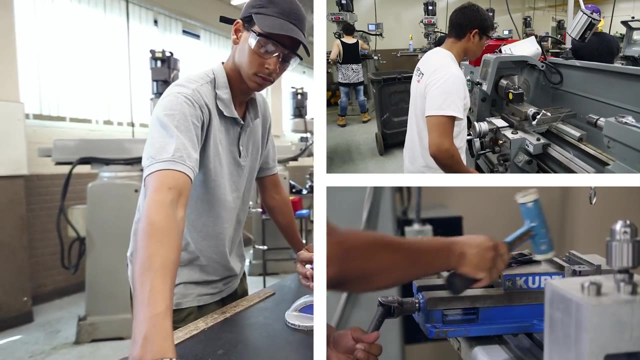 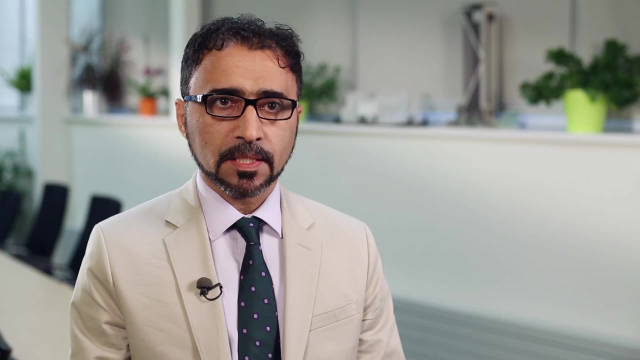 My experience at the School of Mechanical Engineering Technologies has been awesome. We learned to machine high efficiency parts in the industry. We learned how to fix problems. The main benefits that George Brown provides to our mechanical engineering students is to give them different opportunities, either as co-op or as capital projects or applied. 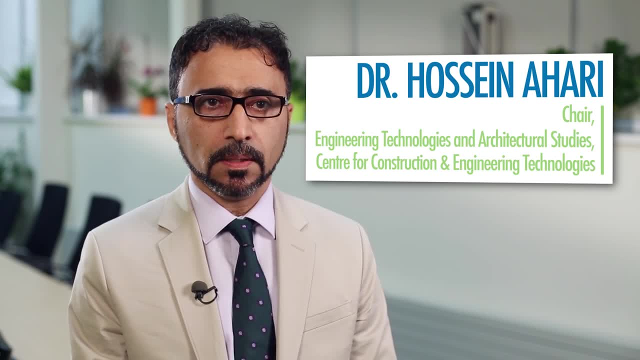 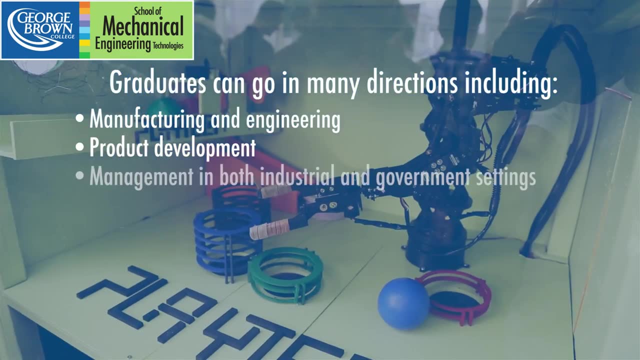 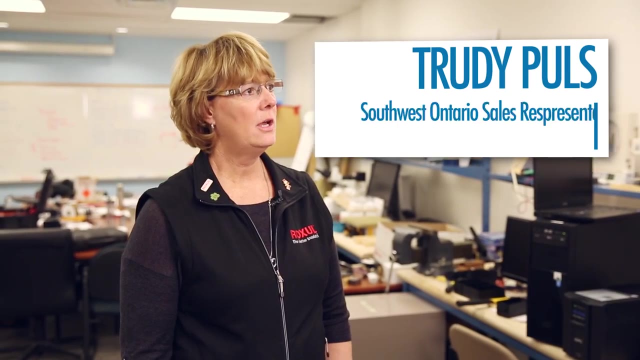 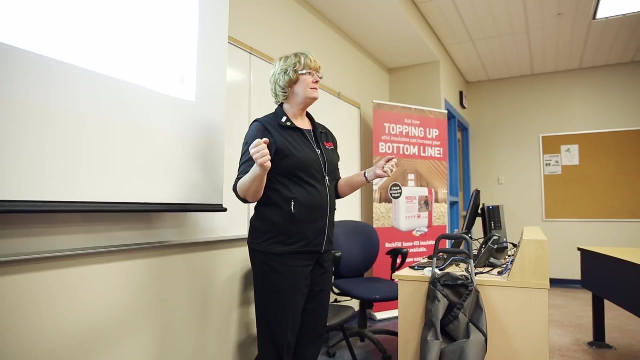 researches, that they can get involved to gain that hands-on experience which help them to just be ready to work when they graduate. There's lots of talent at George Brown College and, as an industry leader, we will look to hire George Brown students if the role fits. 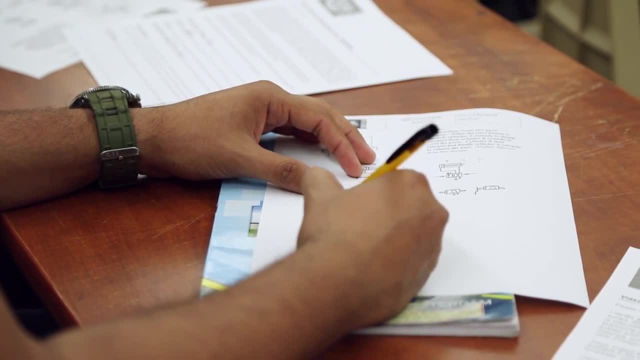 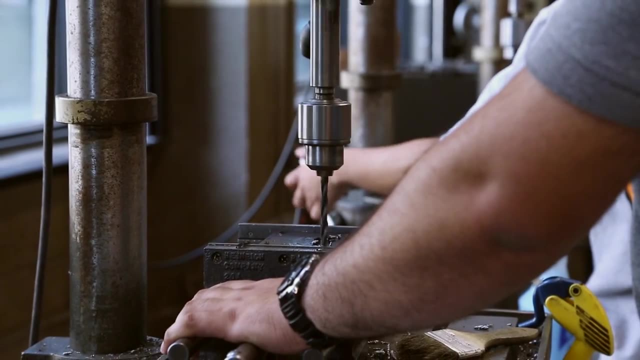 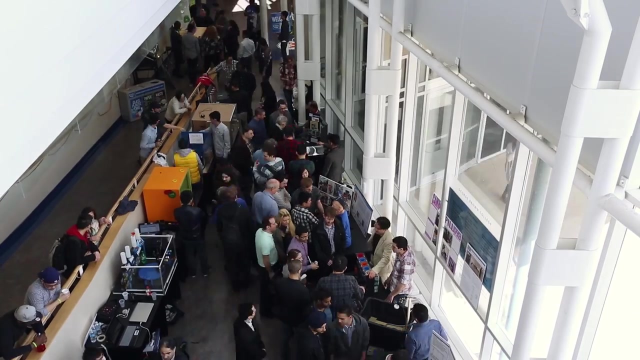 They're successful candidates and they're really adding to our team in a positive way. So programs in Mechanical Engineering Technologies School are very close together and a student can change their past face later on after entering the college. Department of Aerospace in the University of Toronto has annual projects. 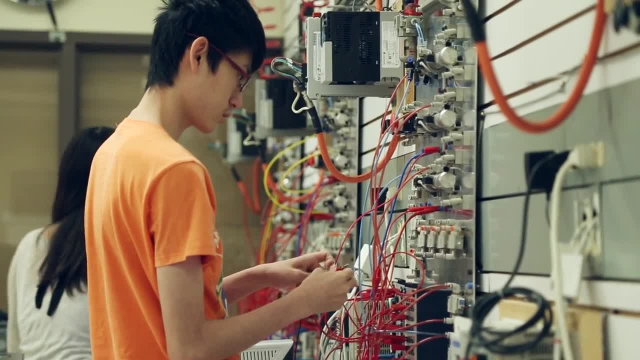 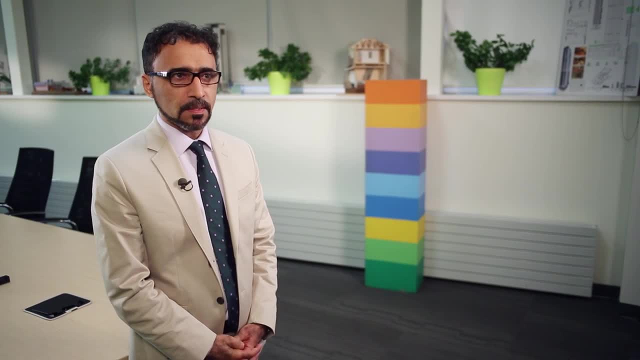 We had the collaboration with U of T on making those parts for them, So they normally provide us with the design and we have data students working with our students here, under the supervision of our faculty, to actually bring that design to life and make it happen. 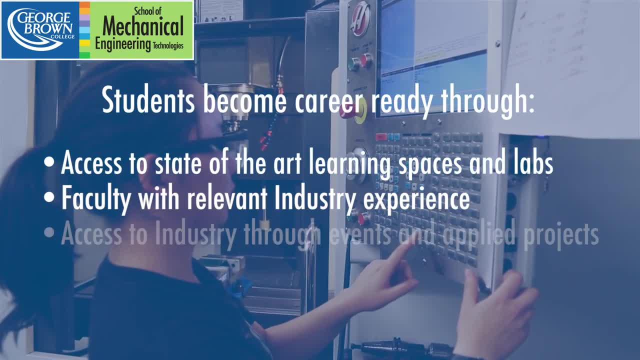 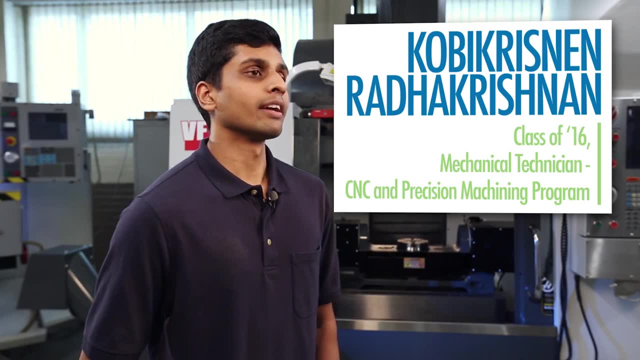 That's part of our jobs. The biggest learning experience for me was learning how to use the machines, Being able to get on the CNC machines and knowing how they work, knowing how to set tool offsets and setting tools into the machine, because that's a big thing that people do. 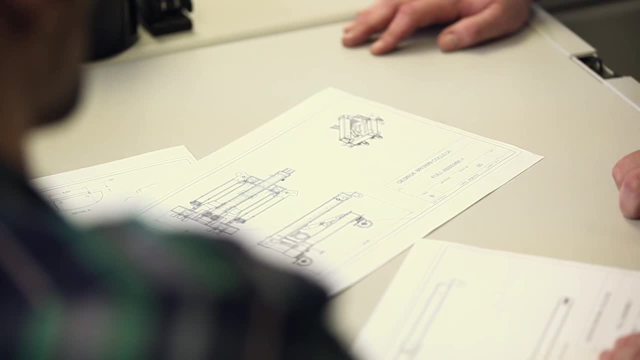 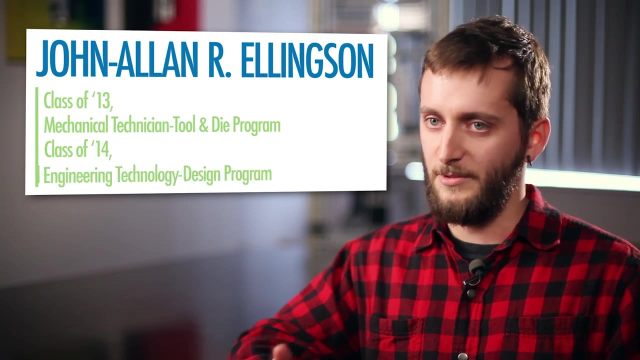 in the workplace. now Our design projects. we come up with a basic design for something and then, as an engineer, the next thing you do is you go to catalogs. Inevitably something doesn't fit because you didn't realize something. so there's a kind 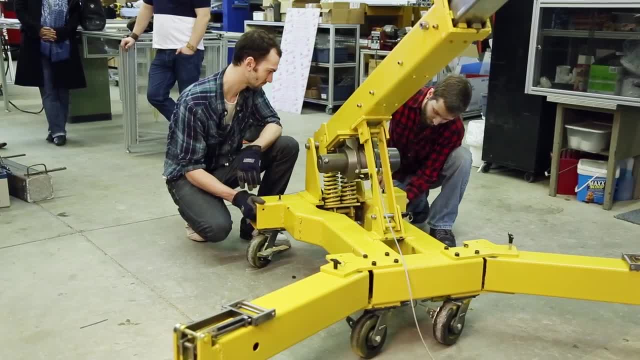 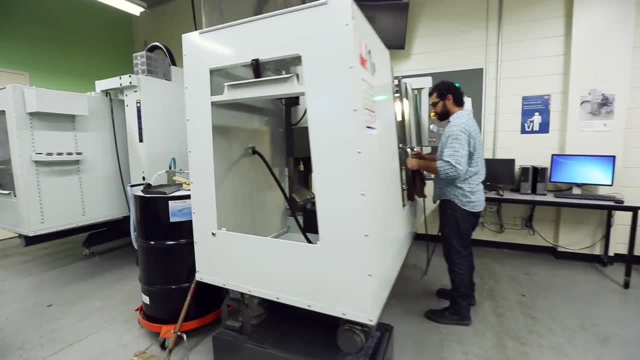 of learning process there that's cumulative, Then the next project. you're not going to make that mistake. If George Brown can provide experiences like this, then that really gives them a leg up. I was working on cutting edge technology. These are new machines that we're working on with new tools, so I really got to see. 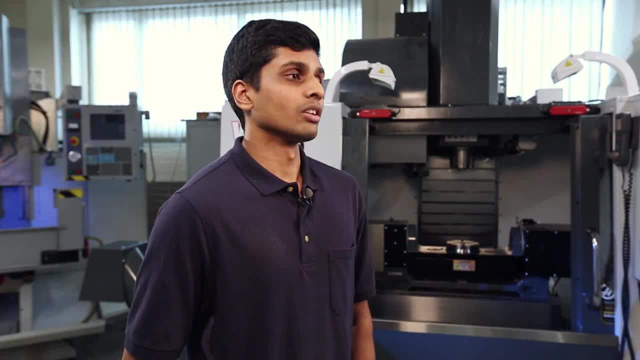 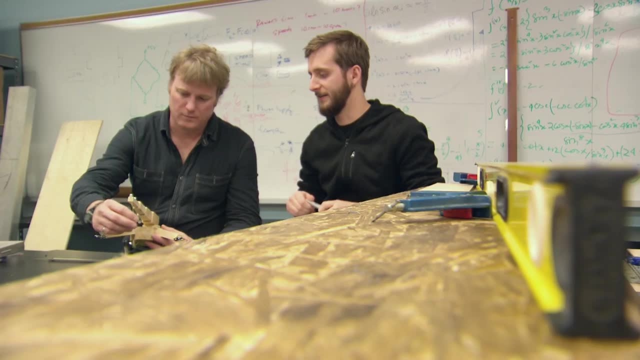 what people in the industry were using. and also I really enjoyed learning about these machines from my professors. They were really good, They really were more supportive and they took an interest in the students who really wanted to learn things. The faculty at George Brown kind of gave us all these different experiences from different